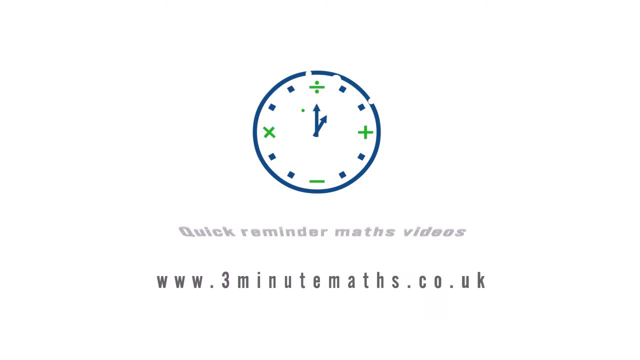 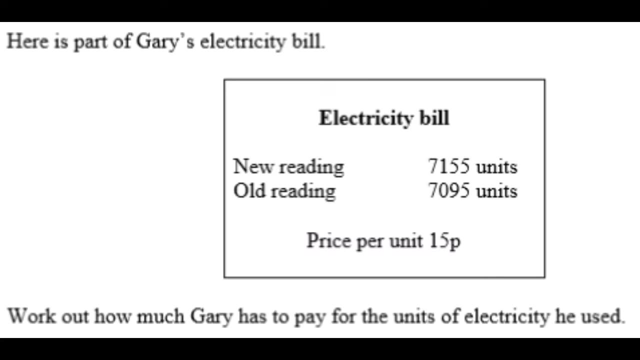 Hi. so this particular playlist is all about answers to tough questions, and the whole idea is that I'm going to post the question If you pause the video, have a go at the solution, and then the answer will be given in the final part of the video. I hope it's useful to you. 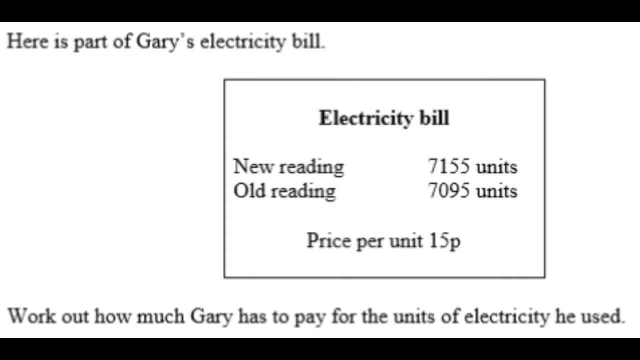 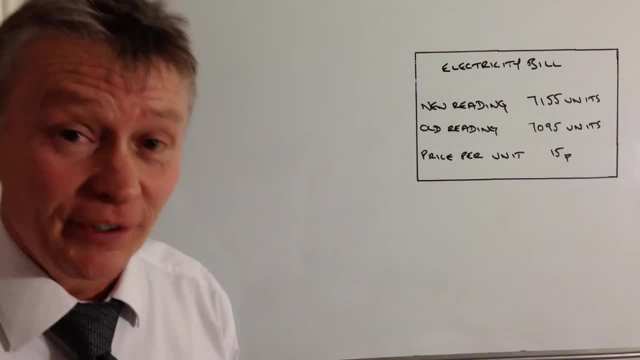 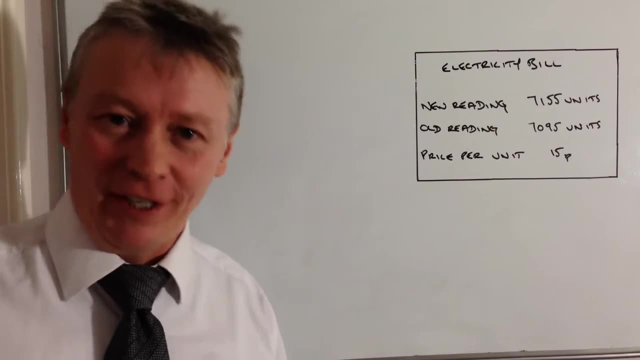 and please do add a comment like subscribe to the site and I'll look forward to seeing you inside the next videos. Hi, so in this particular video. this is the fourth video in the series on functional maths. It's basically relating to real life situations. This one's fairly straightforward and this 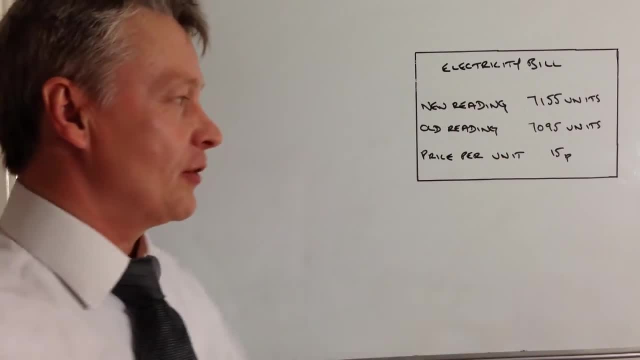 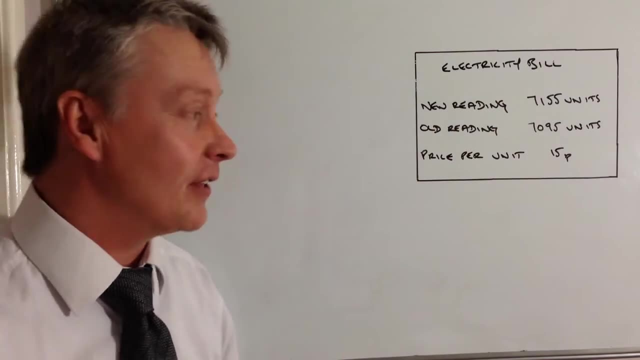 particular person is paying a price per unit on his electricity bill of 15 pence and he's had a reading and a new reading of 7,155 units and his old reading 7,000.. The basic question is: how much does he pay? You need to maybe follow the link below in. 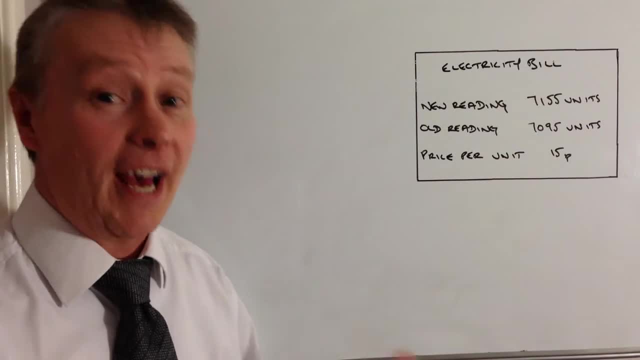 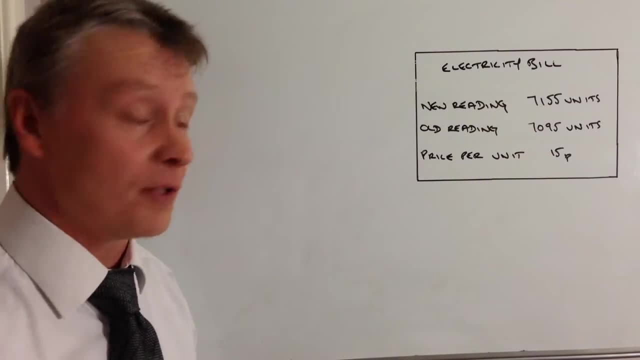 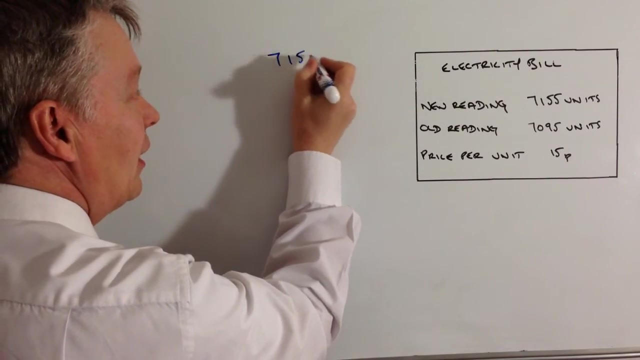 the description, You'll be able to download this particular question and all the questions in this particular playlist. Okay, so we need to work out how many units he's actually used between the old reading and the new reading. So it's a fairly straightforward takeaway. We've got 7,155,. take away 7,095.. 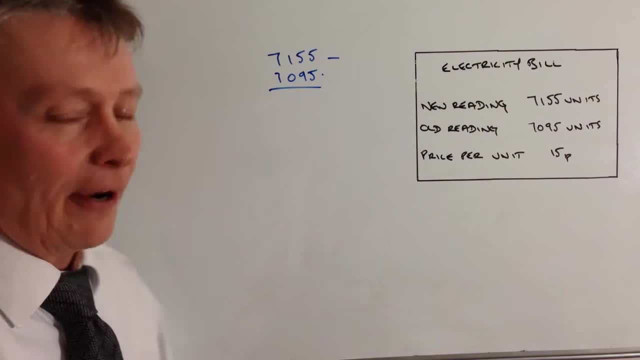 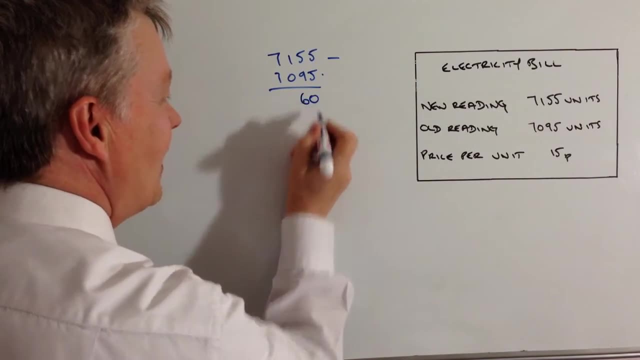 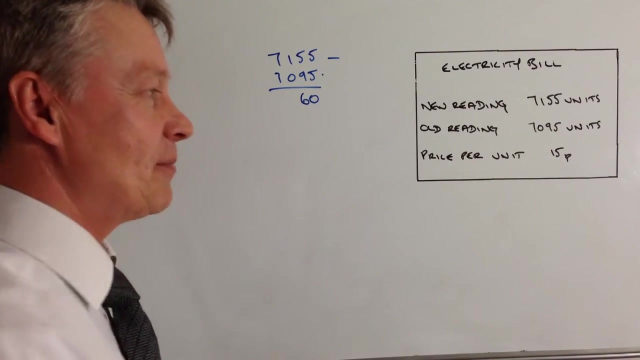 So, however you do that- and I'm very aware that there are different methods of doing these sorts of takeaways- but that will work out at 60 units for you. Okay, so this particular person's used 60 units and the price per unit is 15p, so all. 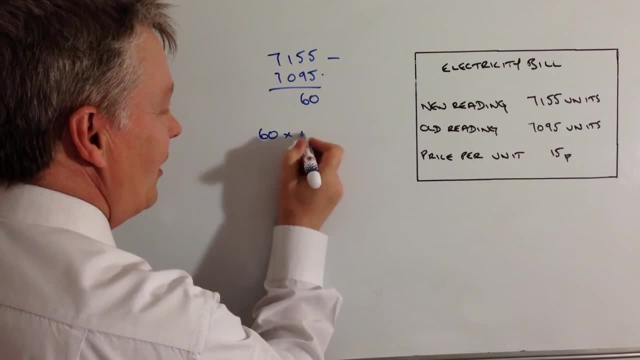 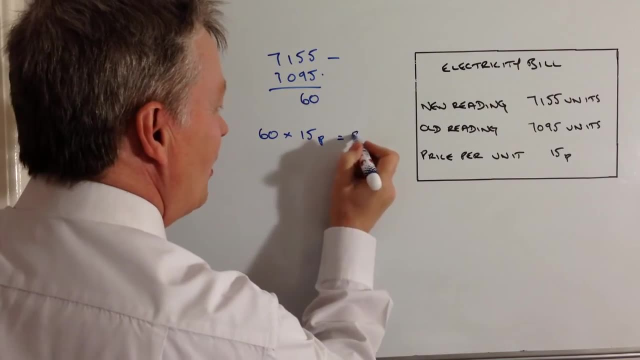 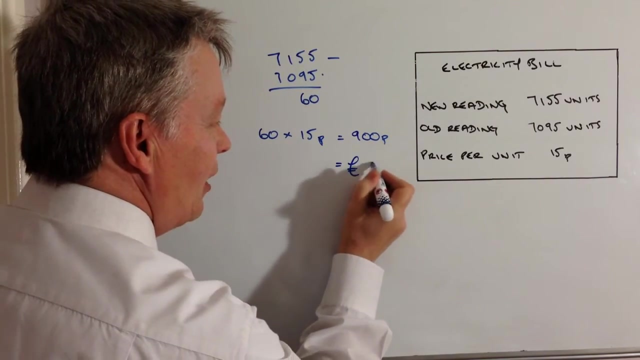 we're gonna do is multiply 60 times 15 pence. Okay, now that's going to give us the equivalent in pennies, which is 900 pennies, And we need to convert that through to pounds, because the question usually will ask. 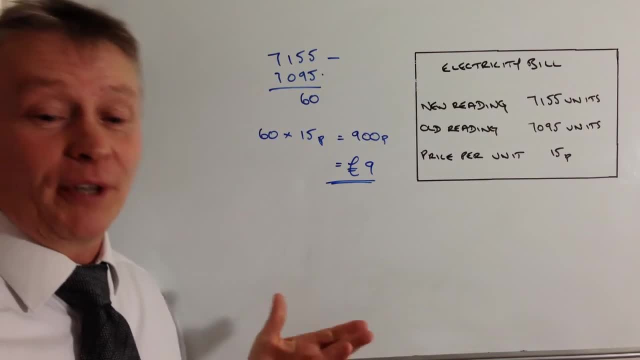 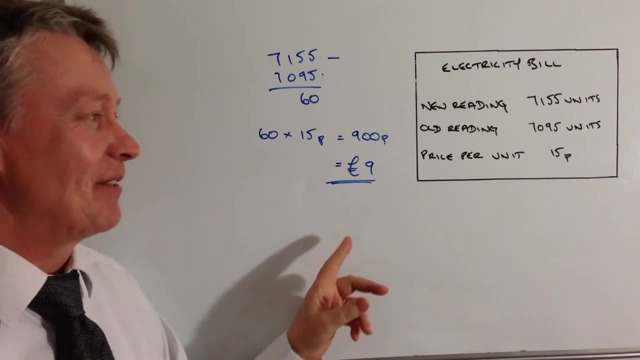 for a pound answer of nine pounds. So this particular person's paying nine pounds for this bill. Now I've got to say in the UK that would be considered very, very cheap indeed, But nevertheless, that's the question. I hope that's been okay for you.